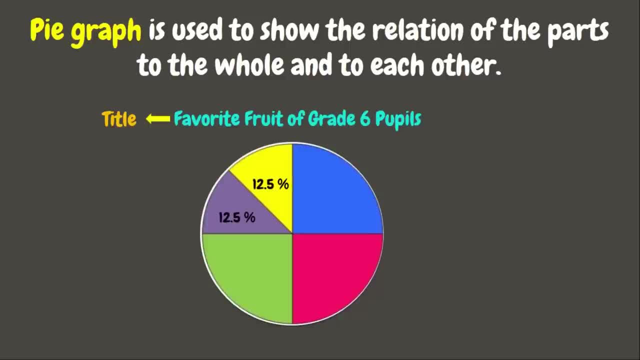 item. The percent which shows what part of the whole is being represented is called sector, while the names of the items or categories are the labels, which can also be shown in the form of a legend. Now that you already know what a pie graph is, let us make a pie graph. 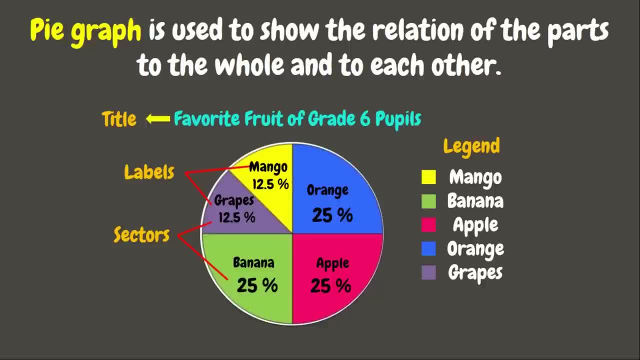 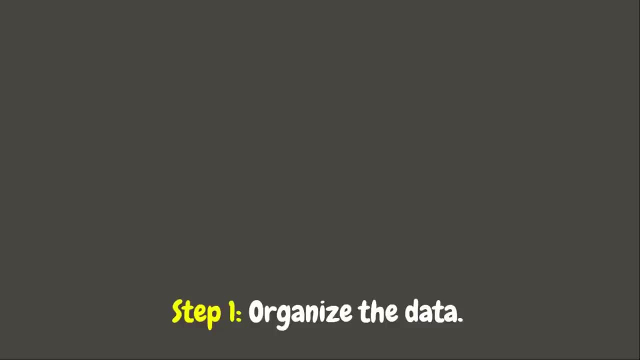 Let's start. Let's start. First step that you need to do is to organize the data. You can organize the data by drawing a table. We need to determine the important facts that you would want to see in your graph From our problem. Santa's family would want. 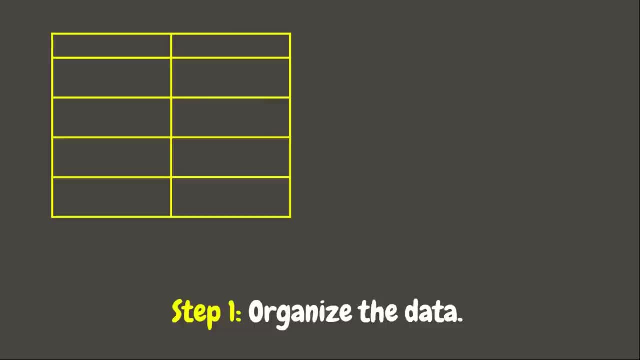 to make a pie graph of their weekly expenses. Therefore, for our first column, we are going to list all the expenses- Oh Congratulation- which are food, light and water, transportation and miscellaneous. For the next column, let's put the corresponding amount spent for each item. 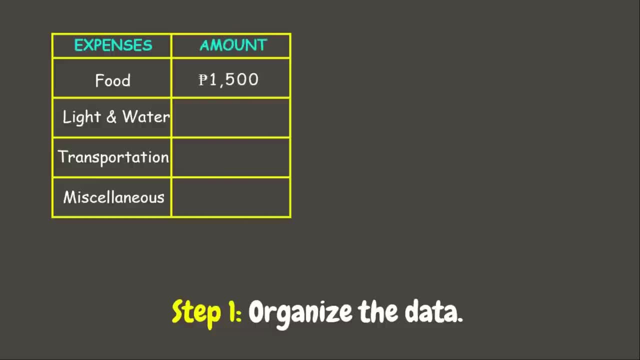 For food we have 1,500 pesos, 600 pesos for light and water, 300 pesos for transportation and 600 pesos for miscellaneous. Now for our next step. we need to convert each amount into percent to determine what part of a whole each item represents. 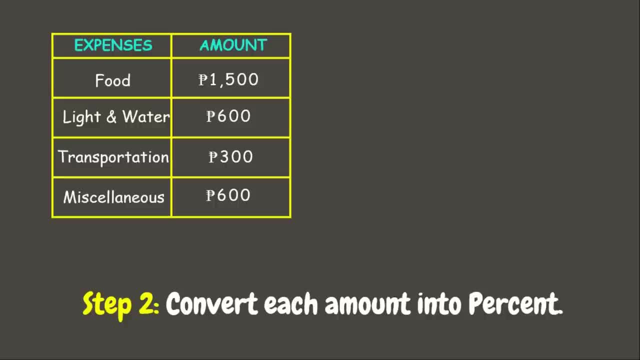 But first we need to get the total amount spent for the expenses. Let us add: We have 3,000 pesos. Now let's add another column for the percent. There you go. To convert each amount into percent, we need to divide the quantity or the amount of each item by the total quantity or amount and multiply it to 100.. 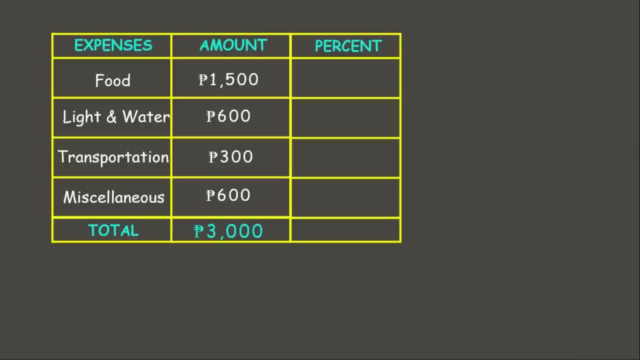 Let us try First. let's have food. The amount spent for food is 1,500 pesos divided by the total amount, which is 3,000 pesos. Let's divide. Since 1,500 is smaller, let us add 0.0.. 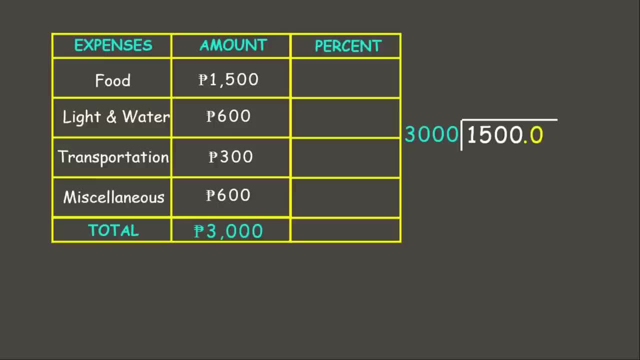 There. Now we have 15,000 divided by 3,000 and that is 5.. And let us put the decimal point aligned from the dividend. Now, 5 times 3,000 is 15,000, and if we subtract this that will be 0.. 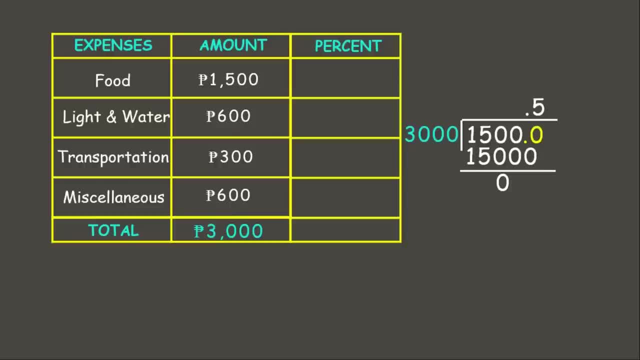 Now we have 0.5, multiplied it to 100, and that will be 50%. Now that is the percent for food. Next, let's have light and water, which is 600 pesos divided by the total amount, which is 3,000 pesos. 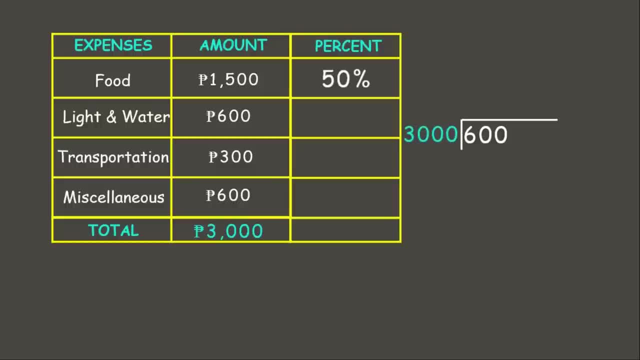 Again, since 600 is smaller than 3,000, let us add 0.0.. So that would be 6,000 divided by 3,000, which is 0.2.. 2 times 3,000 is 6,000.. 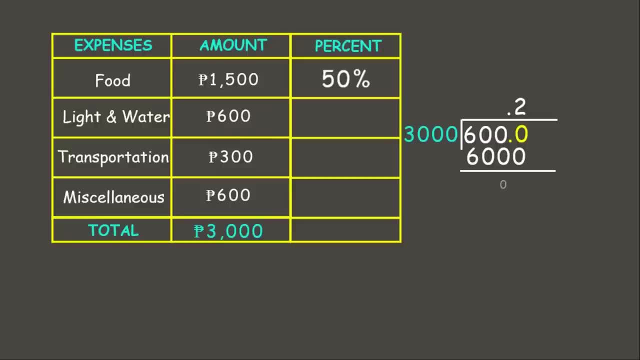 And if we subtract this, this will be 0.. Now we have 0.2 times 100 is 20%. Great job, Now. that is the percent for light and water. Now let's move on to transportation, which is 300 pesos divided by the total amount, which is 3,000 pesos. 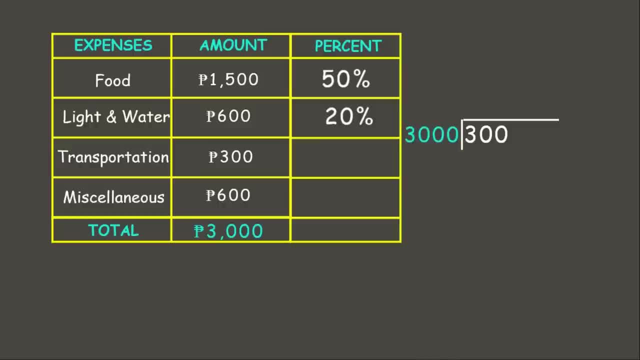 Since 300 is smaller than 3,000, let us add 0.0.. Now we have 3,000 divided by 3,000, which is 0.1.. 1 times 3,000 is 3,000, and if we subtract this, this will be 0.. 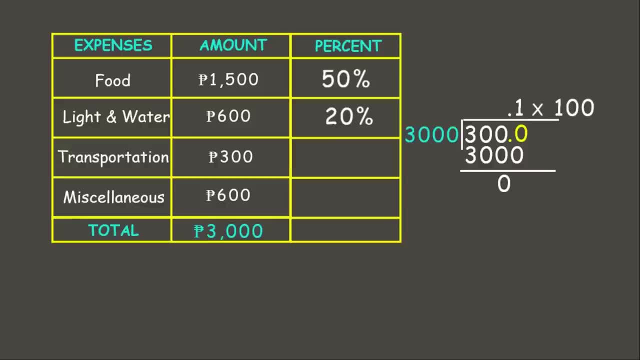 Now we have 0.1 times 100 and that is 10%. Now that is the percent of transportation- Awesome. Lastly, we have the miscellaneous, which is 600 pesos and just the same as the light and water. It means that they have the same amount of money. 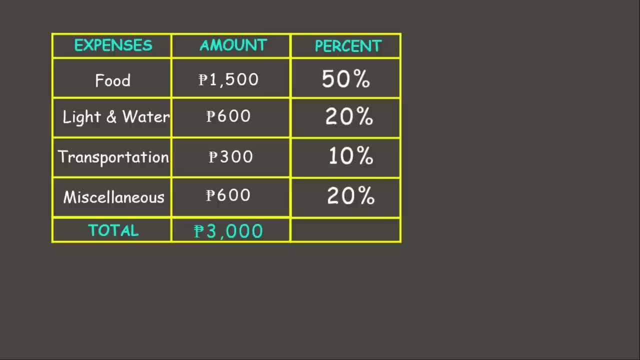 It means that they have the same amount of money, They have the same percent, which is 20%. Now this is a total of 100%. Now the third step is to compute the number of degrees per item. This is to determine how are we going to accurately cut or divide the circle. 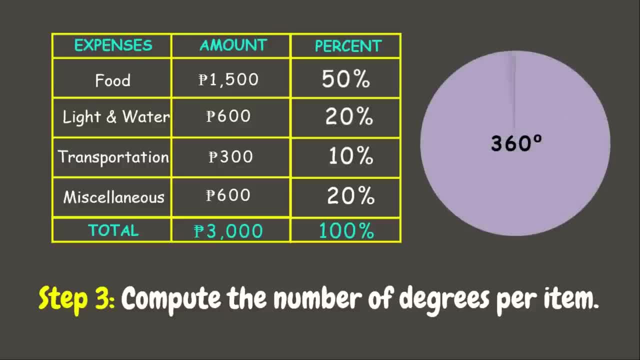 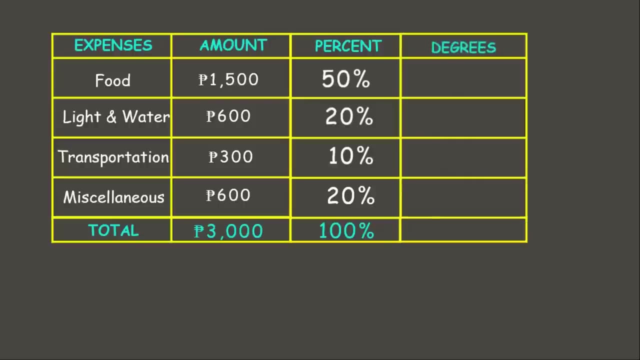 We all know that a circle has 360 degrees And to get the degrees for each item, we just simply need to multiply 360.. 360 degrees to the percent of each item. Let us try First. let us have food. We have 360 degrees times the percent of food, which is 50%. 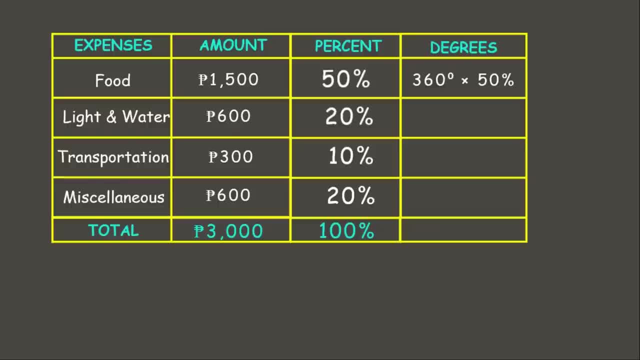 First we need to convert percent into decimal. The decimal form of 50% is 0.50.. Therefore, 360 times 0.50 is 180 degrees, Since 50% means half and half of 360 is 180. next we have the light and water, so that would be 360 degrees. 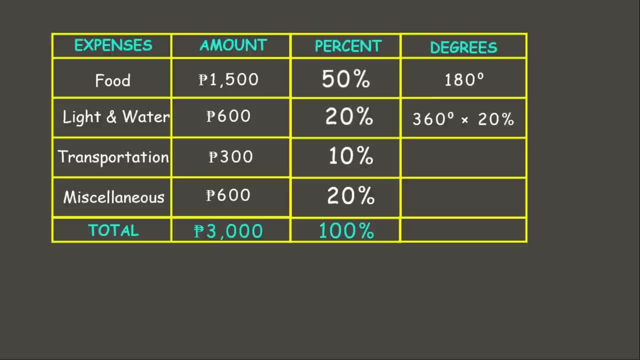 times 20 percent. the decimal form of 20 percent is 0.20. 360 times 0.20 is 72 degrees- wonderful. next we have transportation, which is 10 percent, so that would be 360 degrees times 10 percent. the decimal form of 10 percent is 0.10, so that would be 360 times 0.10, which is 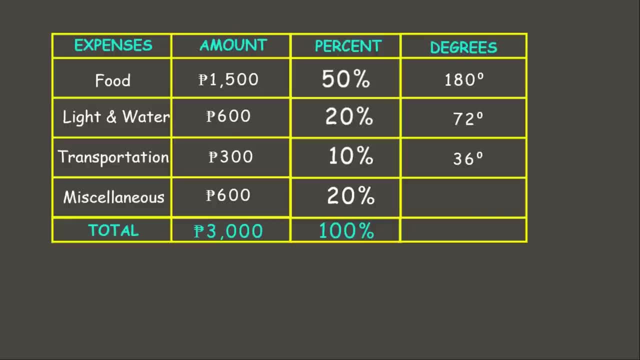 36 degrees. and finally we have the miscellaneous, which is also 20 percent. we have 360 degrees times 20 percent and the decimal form of 20 percent is 0.20. therefore, 360 times 0.20 is wonderful. it is 72 degrees, which is a total of 360 degrees. 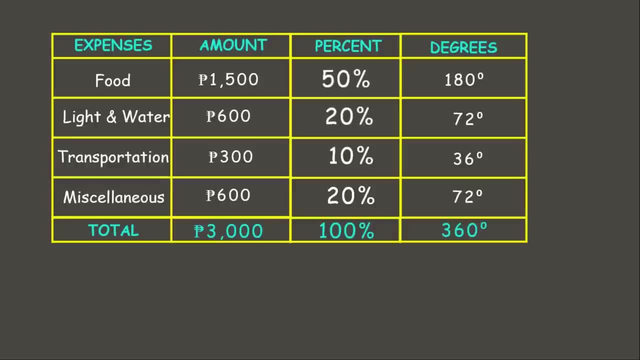 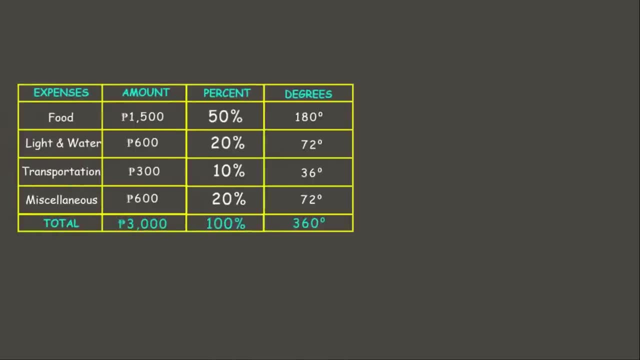 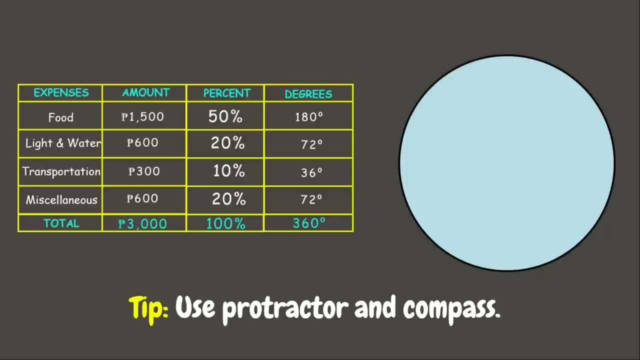 and now that we already have our needed data, it's time for our next step, which is to construct the pie graph. in constructing a pie graph, let us first draw a circle. one tip is to use the protractor or a compass to accurately divide the circle according to the degrees of each item. 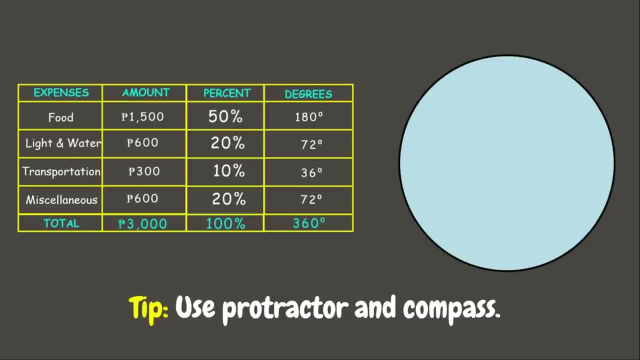 but we can also do some estimation if protractor is not available. for example, we have 180 degrees for the food, which shows fifty percent of the whole. since fifty percent means half, it simply means that we can already divide this circle into half, and this will be the part for the food. 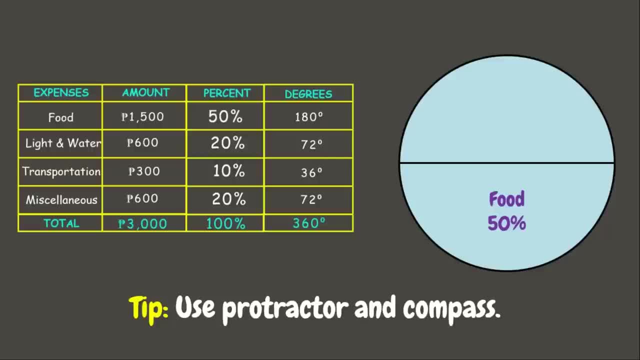 next, for light and water. it is 72 degrees, or 20 percent of the whole. let us use a protector with this one. let us start from zero, then mark until 72 degrees. here we have 70, and let's just add two lines to that will be 72 degrees. there you go. now that is light and water, which is 72 degrees. 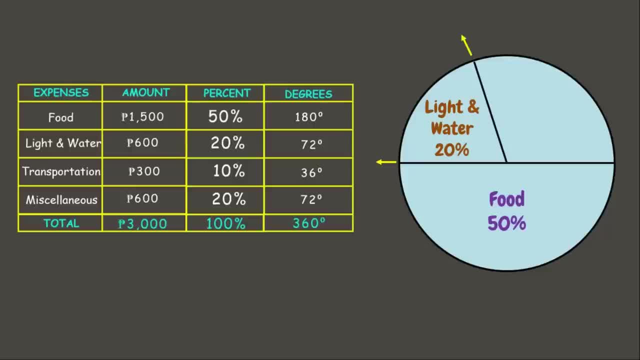 or 20 percent of the hole. next let's go to transportation, which is 10 or 36 degrees of the circle. again, let us use a protector with this one. so let's start again from zero and count until 36.. here we have 30, so we just simply need to count six more lines. there you go. 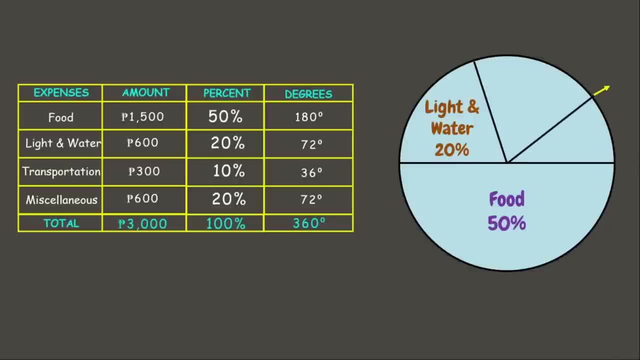 now this is our transportation, which is 10 of the hole. lastly, we have the miscellaneous, which is 20 or 72 degrees. since we have one last left, the remaining part of the pie graph will automatically be the miscellaneous, which is 20 or 72 degrees of the circle. great job, now for our final step. 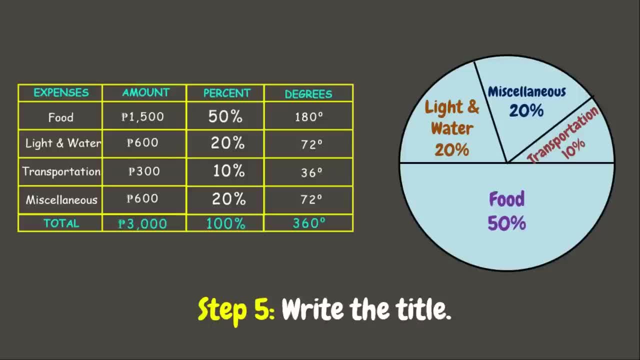 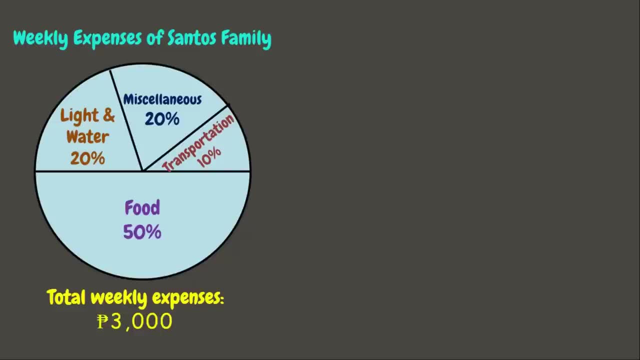 don't forget to write the title. the title of the screen is the weekly expenses of santa's family. awesome, now that we already done with constructing the five graph, it's time to interpret it by answering some guide. question. number one: which item has the biggest allocation? here we can see that the biggest portion of the hole is food, which is 50. 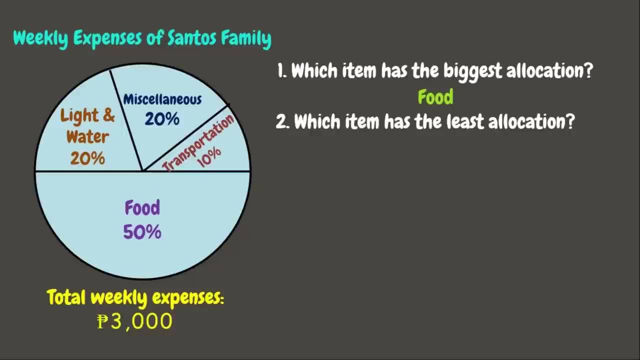 of the expenses. let's have number two. which item has the least allocation? number two: which item has the least allocation? the highest parents allocation lees in the item. It's obvious that the transportation has the least or smallest amount of allocation, which is only 10%. 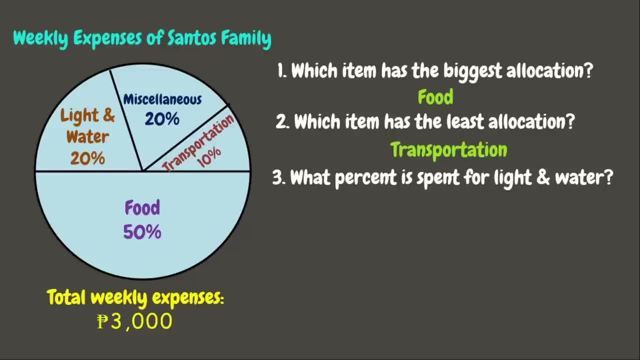 For our number 3, what percent is spent for light and water? It is asking for the percent of light and water, which is 20%. Next, which items have the same amount of allocation? Here we can see that light and water and miscellaneous have the same amount of allocation, which is 20%.